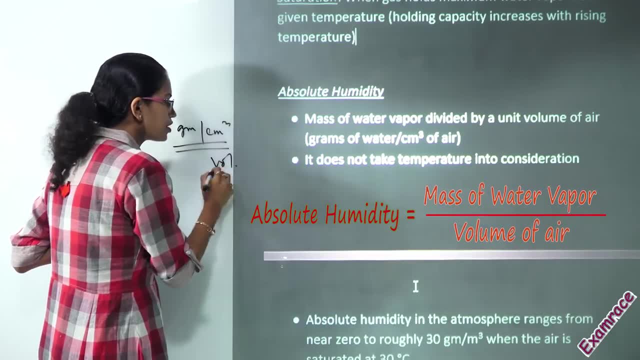 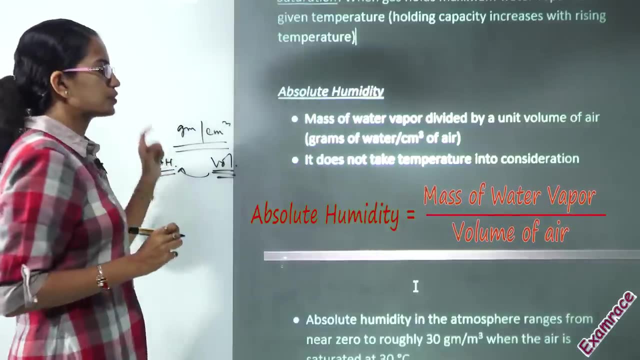 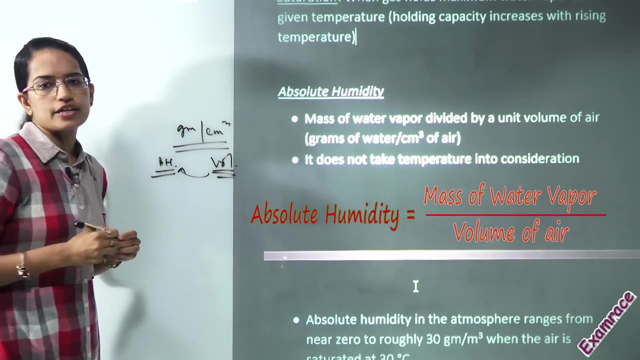 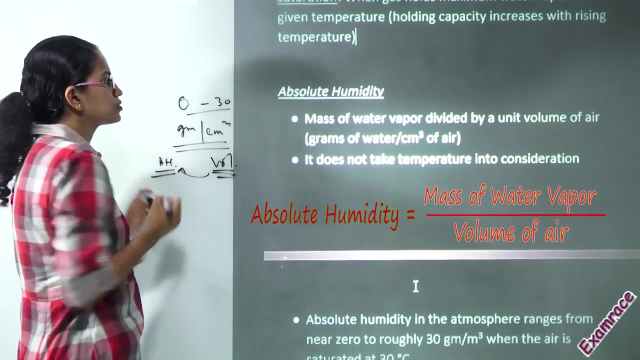 understand absolute humidity. That means if the volume of the air parcel changes, it would affect the absolute humidity and therefore absolute humidity is accounted by the changes in the volume of the air parcel. However, it does not take into consideration the temperature changes. Now, absolute humidity usually ranges from zero to around 30 grams per centimeter cube at a temperature of around 30 degrees Celsius. that we consider as absolute humidity. 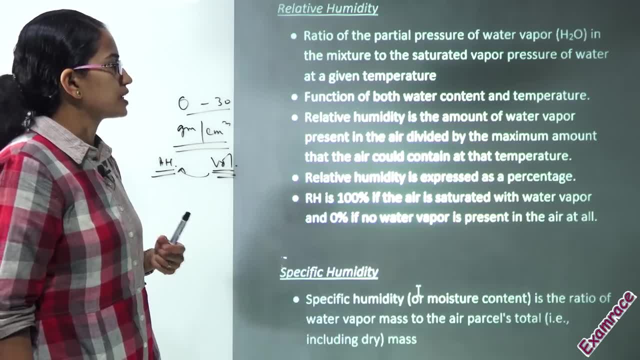 As a basic temperature. The next is relative humidity. Now, since it's relative, it's expressed in percentage. So that's the key aspect here. Now this could be 100%, that means 100% saturation is there, and 0%, that means it is not at all saturated. So relative humidity is expressed in percentage. This relative humidity is affected by both changes in temperature and amount of water content, So it's a function of both the water content and the water properly. 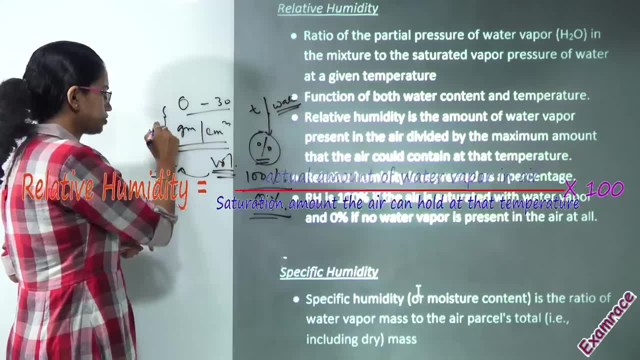 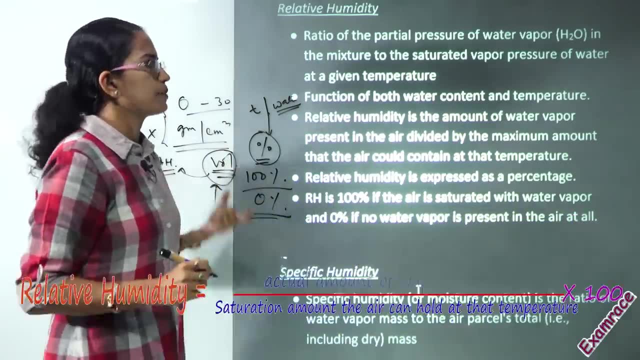 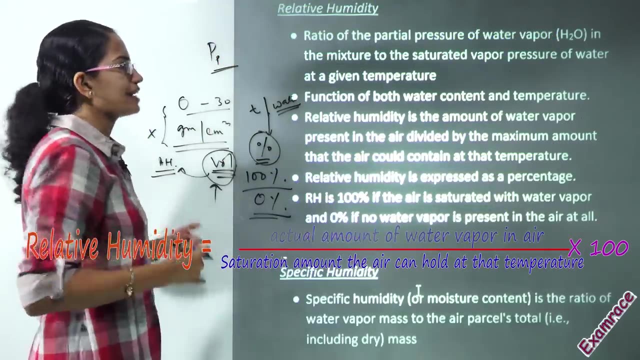 and the temperature that's present. however, absolute humidity was independent of the temperature changes but it varied with the volume that was given. so relative humidity, I can explain. it's the ratio of the partial pressure that's present of the water vapor divided by or present in a mixture, where 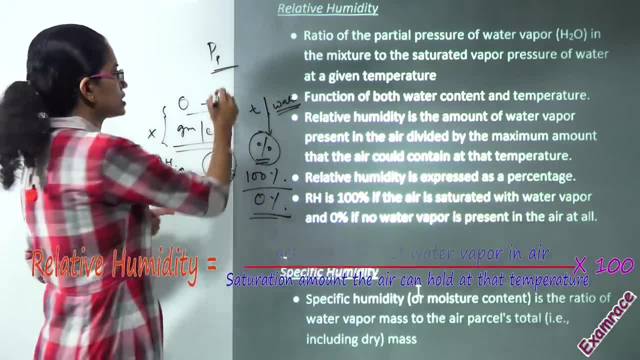 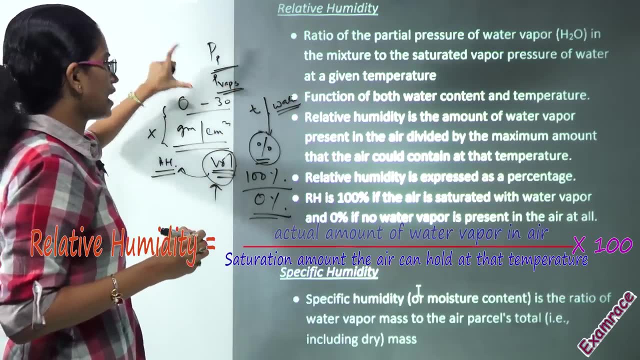 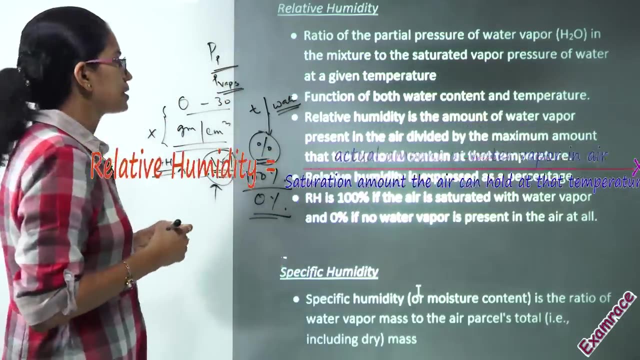 you have a saturated vapor pressure that's given. so vapor pressure for a saturated content that's given would be the base value. so that's how we calculate the relative humidity. the partial pressure divided by the saturated vapor pressure would be the relative humidity the next that we talk. 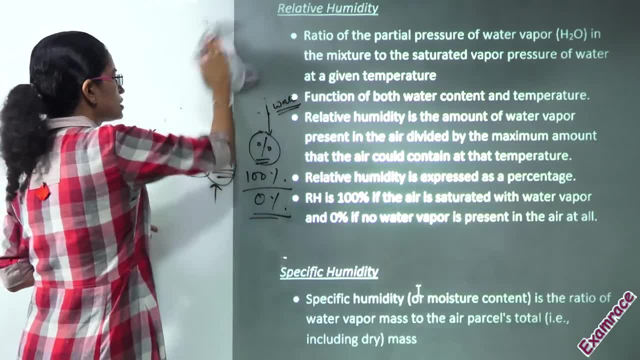 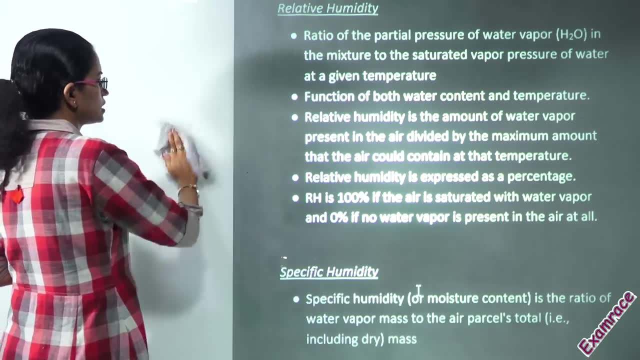 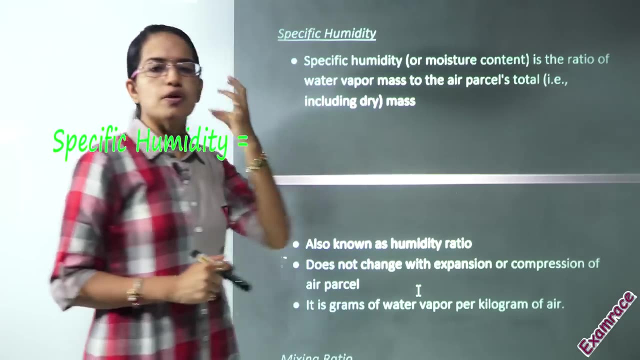 about is specific humidity. now keep a very close eye on what is specific humidity and mixing ratio. a lot of students are confused between the differences in specific humidity and mixing ratio. so when I say specific humidity, I am talking about the ratio of the mass of the air parcel to the total air. 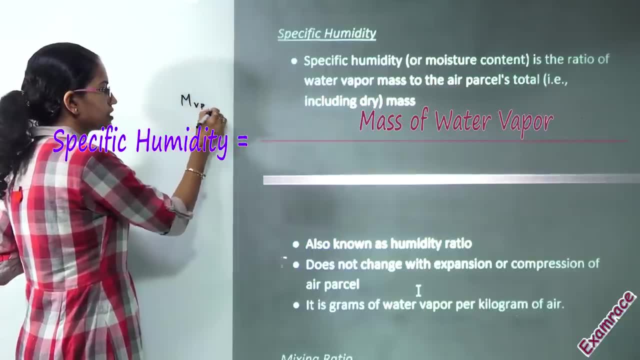 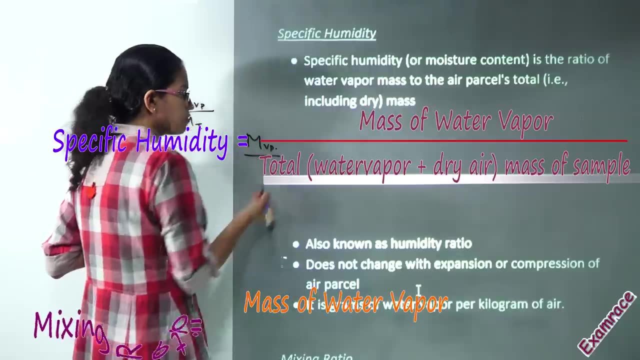 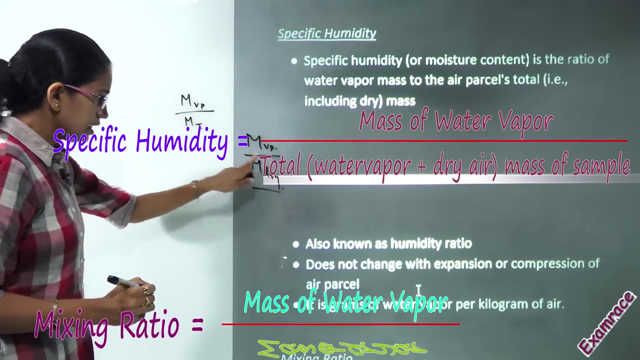 parcel, so mass of the water vapor that's present divided by mass of the total air parcel. however, when it comes to mixing ratio, I am talking about mass of the water vapor divided by mass of the dry air. so that's the key difference. in the case of mixing ratio, the denominator would be mass of the dry air. however, 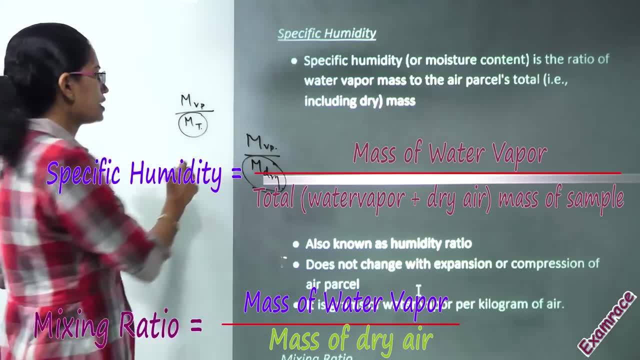 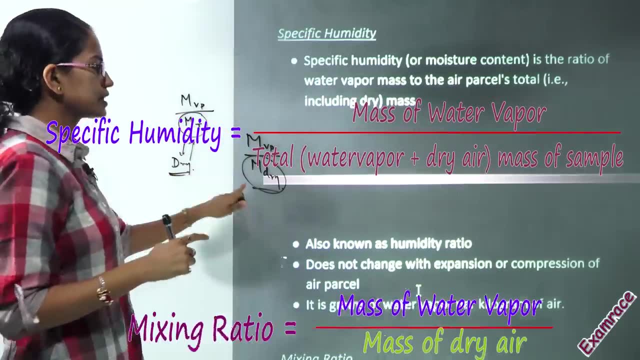 here in a specific humidity, it would be mass of the total air, and this total air mass includes dry mass as well. So here dry mass would be part of it, but here, in mixing ratio, it would be only dry mass that would be considered. So this: